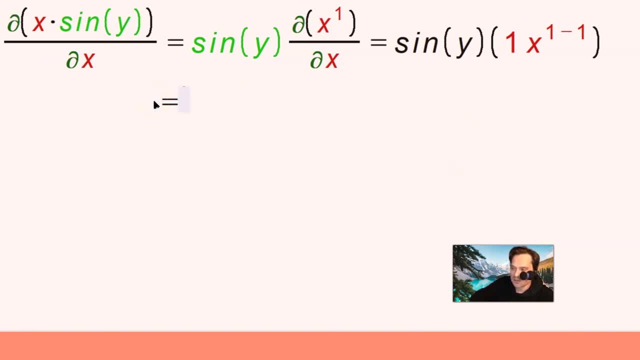 In lower level classes like calculus 1.. Then you finish this up, so you're going to have sine of y. I'm going to make that black now. And this is 1x raised to the 0, so the 0 up here. 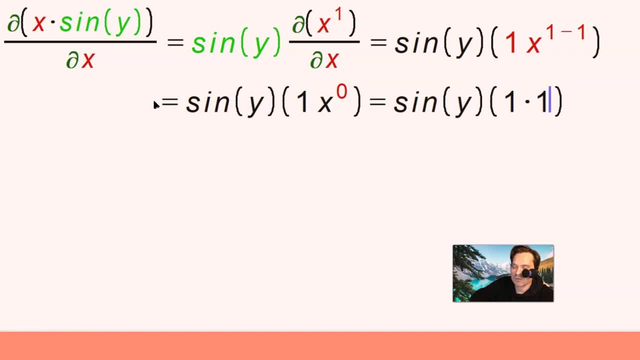 And you think the 0 is 1, so you have sine of y and then 1 times 1. for that reason This part here is like this part here: The green x to the 0 becomes the green 1, right here. 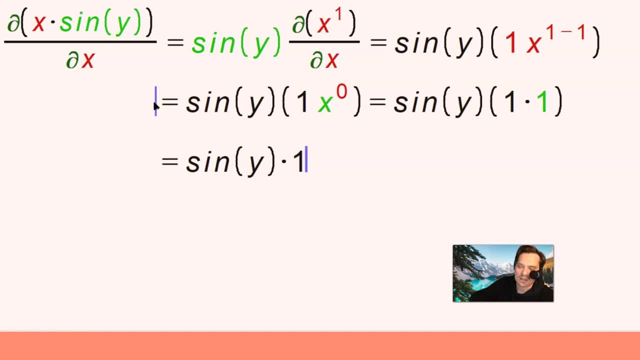 Then you have sine of y. Now, 1 times 1 is 1, so you can write that. And then you have sine of y times 1, which is sine of y. Okay, so this is an example done in great depth. 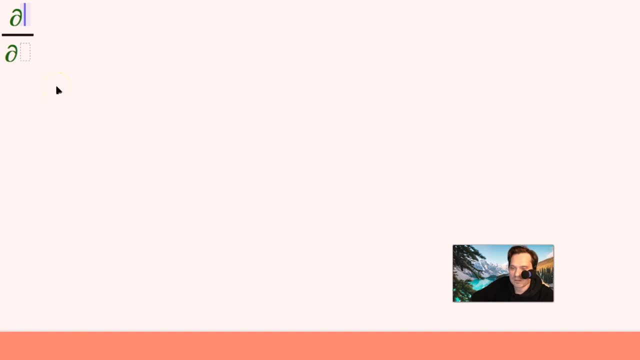 It was helpful. Okay, now let's look at a variation. Okay, so derivative, with respect to x, of x squared and then sine of y. But now let's differentiate with respect to y. So now again, this is y, our differentiation variable. 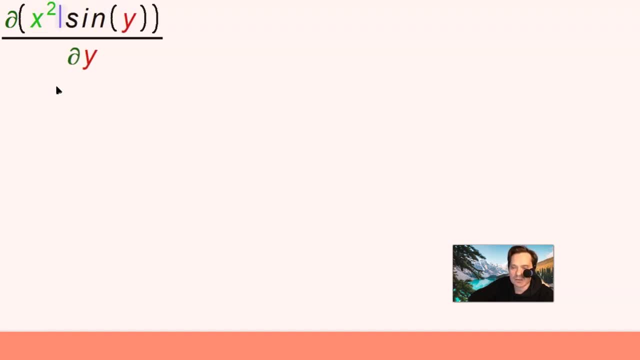 And notice where the y is. The y is now wrapped inside the sine And the x squared here is separate, And this is multiplication right there between them. So for that reason, what you can do is pull the x squared out this way. 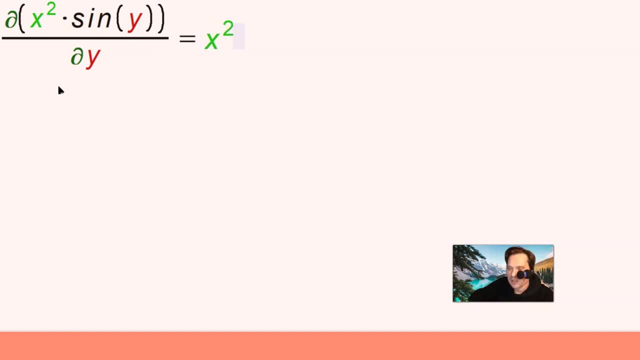 Okay, because it's multiplying sine of y. So pull it out And then what's left over? It's a derivative, with respect to y, of sine of y, like that. Okay, and then y is again here in the bottom. So just keep a careful eye on y right here. 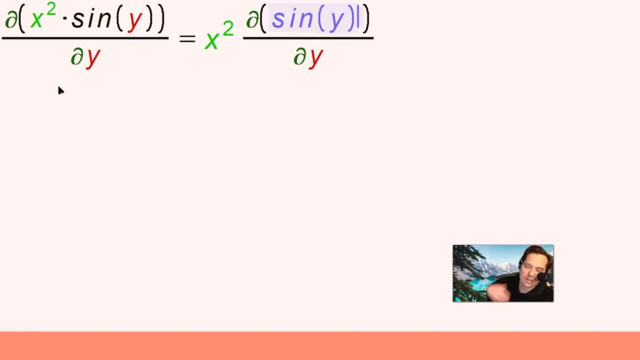 See, For this reason, because y is our differentiation variable, you can not just place the sine of y outside the differentiation operation. It doesn't work like that. You can actually differentiate. So you're going to have x squared. Now. derivative of sine y is just cosine y. 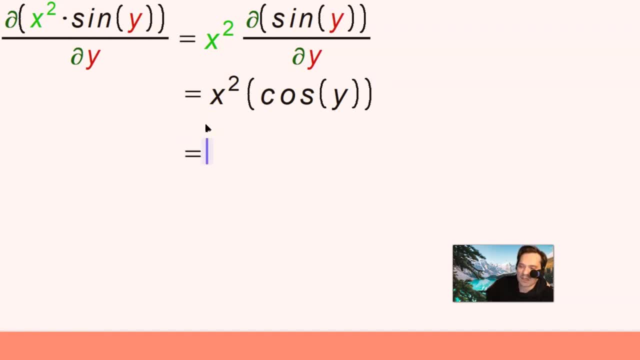 That's really the whole step, if you think about it. But now we just clean this up. So often we just write x squared cosine Y or something along those lines, And that's the derivative. Okay, let's look at the next one. 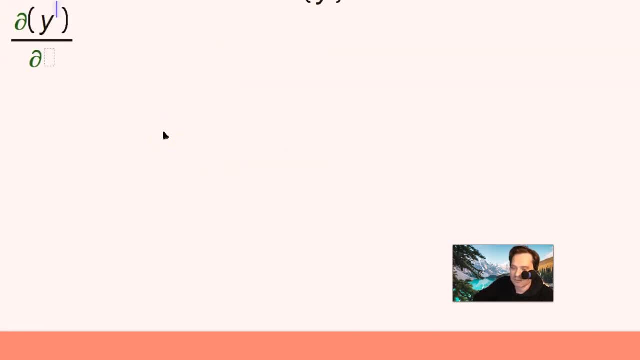 Another variation of this. So now let's do y, say cubed, And then plus x sine y. So again a slight variation, And let's do differentiation here. Let's see, with respect to x maybe. So this is x here. 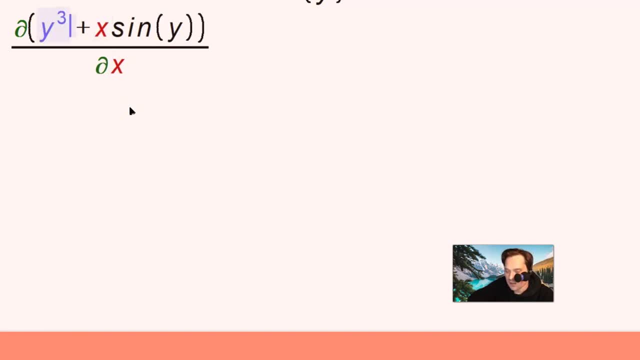 This is x here, Right here. So notice that the y squared part here does not have x in it. So that means this should be seen like a constant, as if it's at 5 or 10. Or 90 or negative 8.. 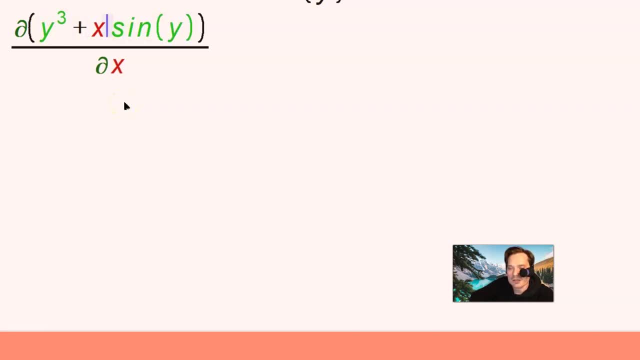 Some number. Okay, the sine y part. again, That is to be seen like a constant with respect to x. So now this one. We can distribute the differentiation operation. So you're going to have y cubed. Now this y cubed, I'll make green. 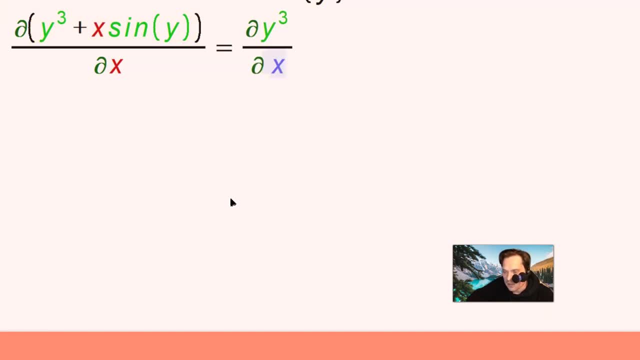 Okay now. the bottom differentiation variable is x. So that's important to understand because look, Y cubed here does not have any x's in it. That means the y cubed is to be treated like a constant with respect to x, Like a number. 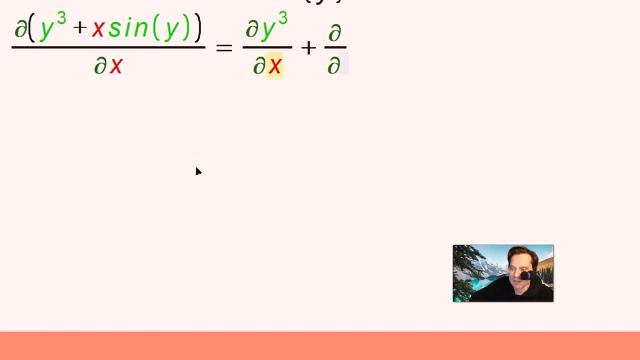 Like 5 or 10 or 90 or whatever, Plus in the partial respect to x. So put the x in here in red X sine of y. So this part again, The sine of y part, I'll make that green. 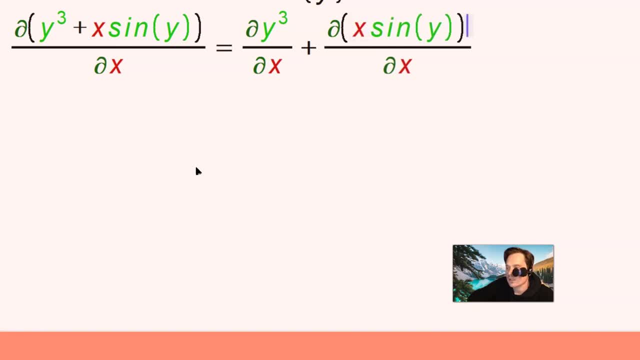 That does not have x in it. The x, however, is present in this position. So when you differentiate, what do you get? Go to the next line. When you do this part, The derivative of y cubed with respect to x is just 0.. 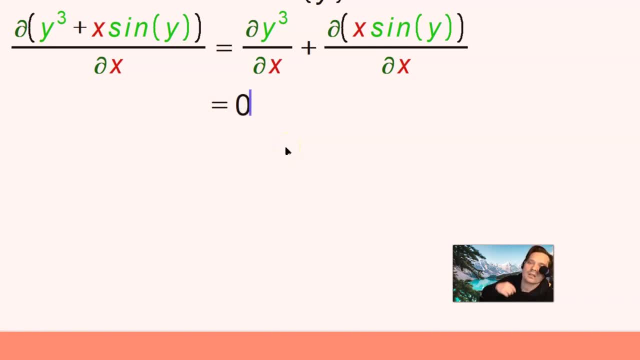 Because the y cubed is to be seen as a constant, And constants have a derivative of 0. They do not change. But now the other part. What it allows you to do is you can pull that sine of y out this way: 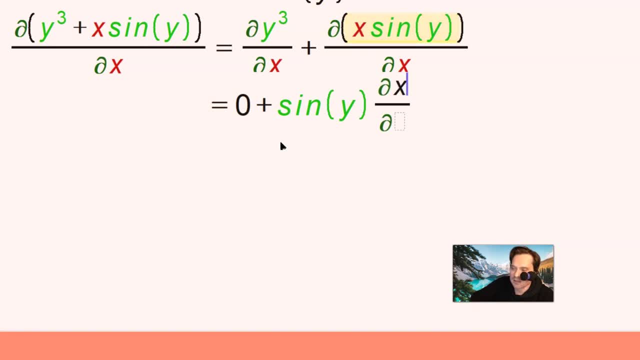 And just multiply by the derivative of that x, Which is really like x, to the first, We call over x Like this. So this is an x And there's an x over here Like that also. So now you simplify, So we have sine of y. 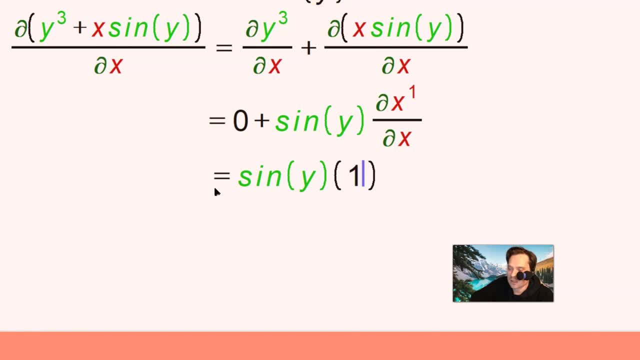 Again, this is green. And then use the power rule, So 1 down, x raised to the 1 minus 1.. And then you simplify this: Sine of y, And then Sine of y. Sine of y, Sine of y. 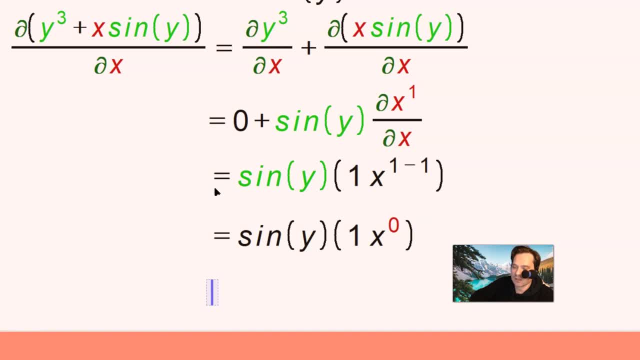 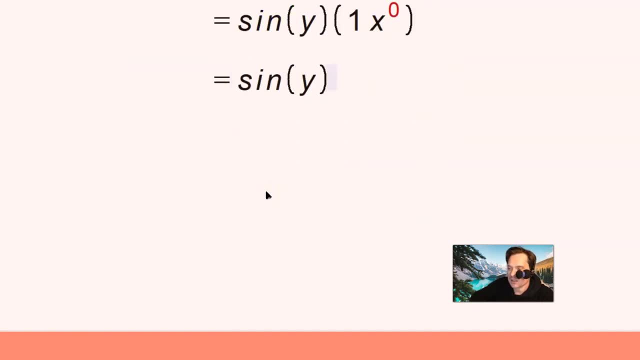 And then Let me pull this up: Sine of y, And this is now 1 times 1.. Because x to the 0 is 1. So you have sine of y times 1.. But that's just sine of y. 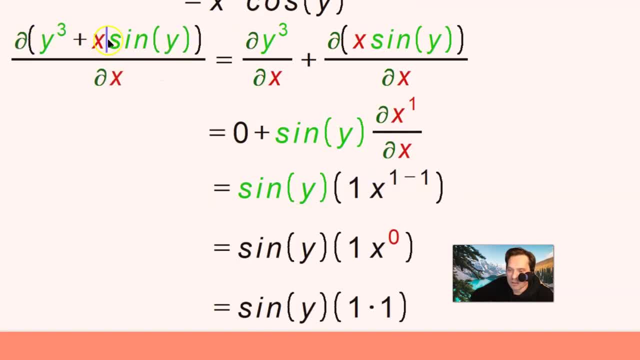 So you see, the result here is the sine of y That we begin with in this position, where it says x, sine of y. Okay, So here's all of our work. This is the first example that I did in great detail. I hope it was helpful.